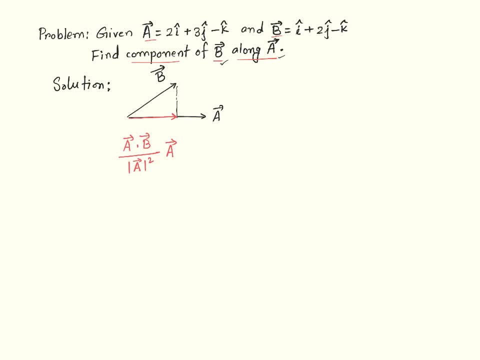 norm of A square, or the magnitude of A square, and then multiply it by the vector A, And that's pretty straightforward. We know how to take dot product by now. So A dotted with B is going to be 2 times 1 plus 3.. 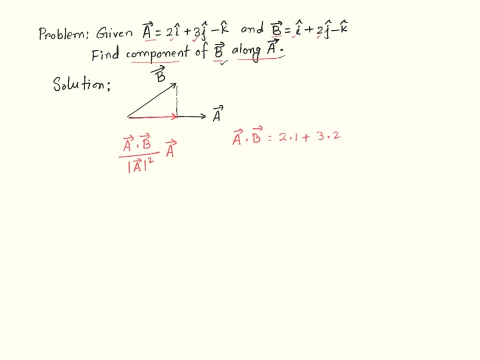 3 times 2 plus negative, 1 times negative, 1. And that's going to give me: 2 plus 6 plus 1 is equal to 8. Actually, 9. That's not 8. So let me just quickly erase it and write: 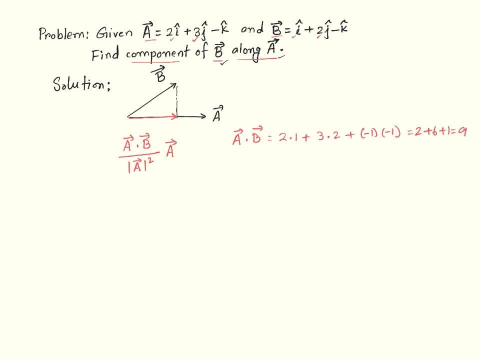 it down 9.. Okay, That's A dotted with B. Now I have to find norm of A square. So which is going to be A square is going to be just so, 2 square. look this: 2 plus 3 square, plus negative. 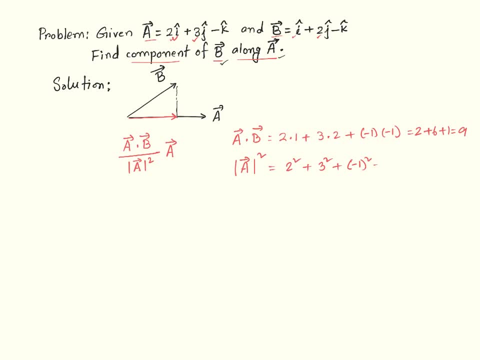 1 whole square, which is going to give me 4.. Plus 9 plus 1 is equal to 14.. Okay, Now I found these two values. All I need to do right now is to take this 9 and 14 and plug it into this formula. If I do that, I'm going. 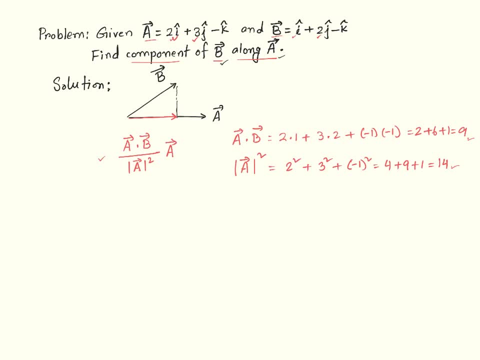 to get the following: A dotted B was 9,, which is this value divided by norm of A square, which is 14.. So I multiplied by 14.. Once again, I got 14.. So I have to figure out how much I need to multiply this number. I have to put it inside. 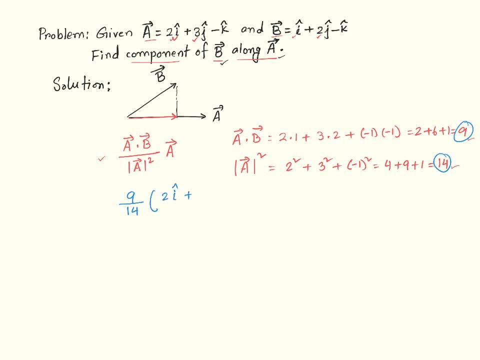 the postcode, And this is going to be 5 times 9 over 14 times 2, which is 2 A plus 2 B minus 2 B is going to be c times minus 7.. Now, now I just need to multiply it out. so 9 over 14 times 2 is going to be 9 over.